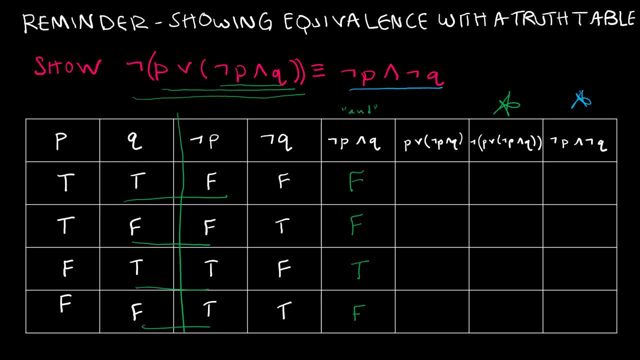 true but that's a false, because I've got one true, one false. Now I'm going to take that new column I just created and I'm going to say P or that new column I just created. So I'm looking at P and the new column and one of them is true, So I'm going to say P or that new column I just 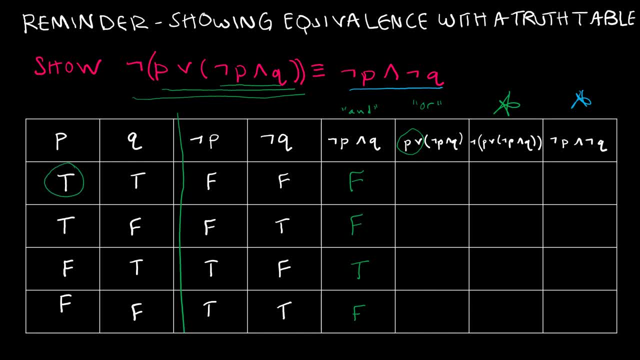 created, and one of them has to be true for me to put a true. So in this row I have a true, so I get a true. And in this row I have a true, so I get a true. And in this row I have a true, so I. 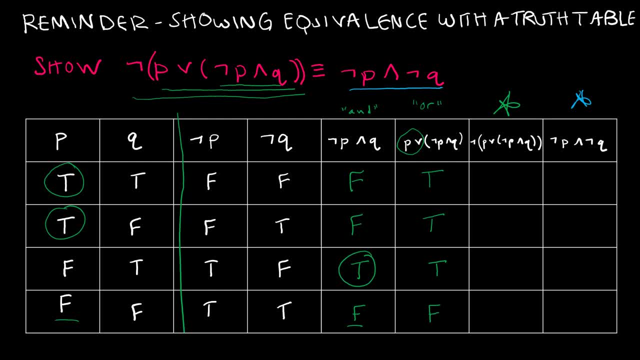 get a true, But in this row I've got two falses, so I get a false. Then my next column is just the negation of that. So that's false, false, false, true. So that's what I'm hoping. my blue column. 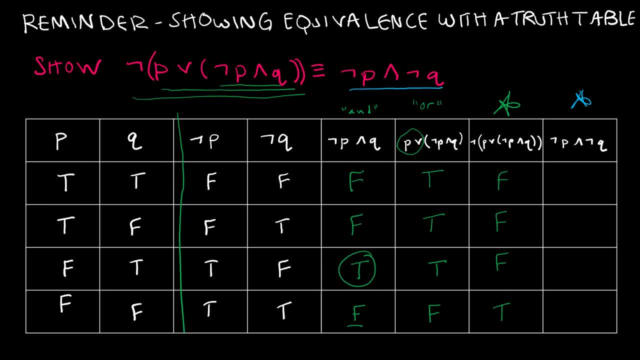 will match up to. So how do I find the values in the blue column? Well, I'm looking at the values in the blue column. I'm looking at not P and not Q. So I'm looking at these two and they both have to be true for me to put a true That gives me a false That gives me a false That. 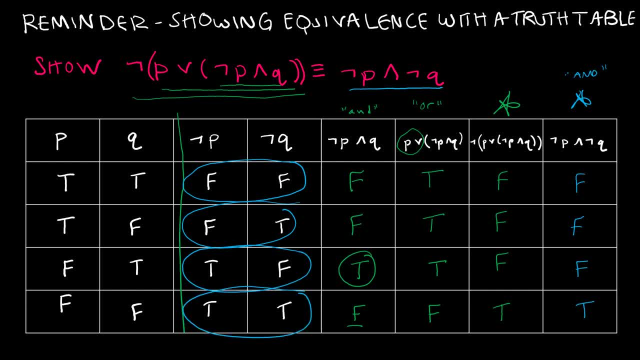 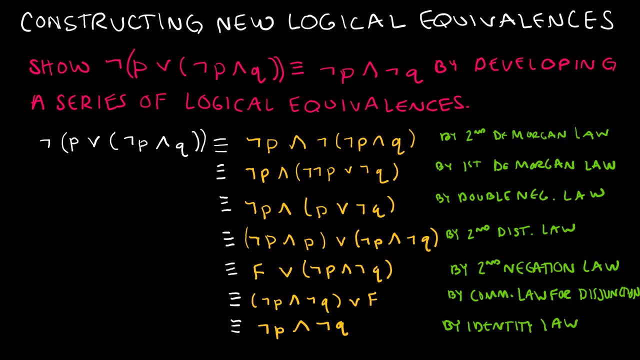 gives me a false, Two trues give me a true. So, as we can see, those two compound propositions are equivalent, which we've shown with the truth table. Now what I want to do is show you another way to prove that. Now I want to take a look at the exact same example and I want to show you how we can construct this. 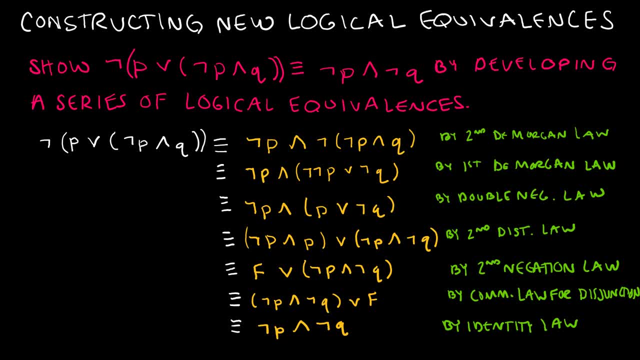 new logical equivalence using things that we already know. So this is going to look kind of like a two-column proof, if you've ever looked at two-column proofs before. But notice, what I'm doing is I'm just proving exactly what I showed with the truth table previously, And when we do. 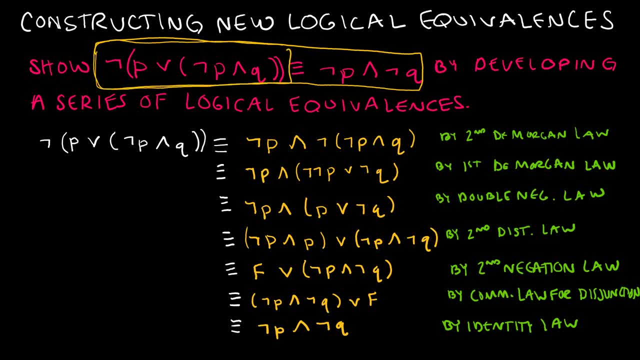 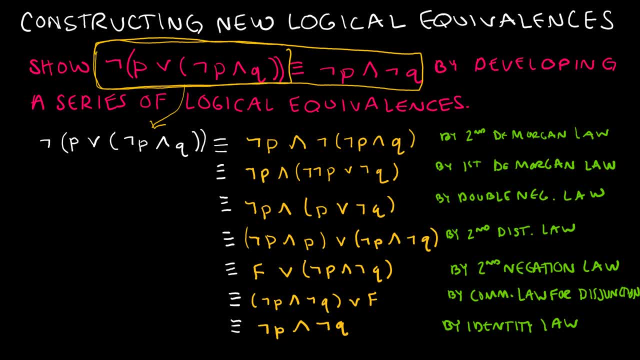 And then on the right side, my goal is some statement that I can use this statement to turn it into based on some law or rule that we know, And I'm going to keep repeating that process until I end up where I'm trying to end up. So this is not something you're probably 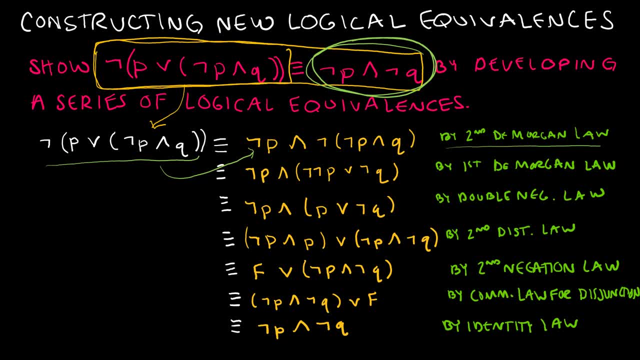 going to be good at right away. to be good at right away, You're going to have to do some practice, But let me kind of walk you through this example, the way that I went through it. So here I have the negation on the outside of 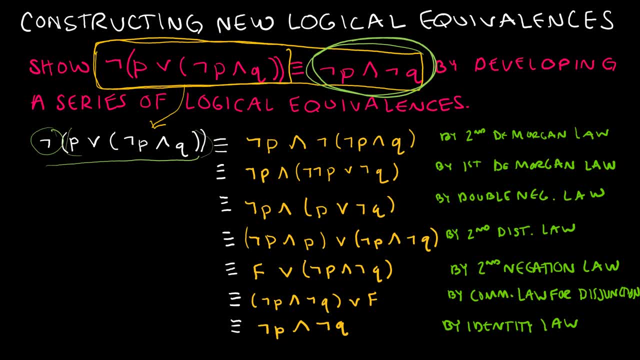 obviously some parentheses, And essentially what I'm doing is using De Morgan's second law, which says if I have the negation of this or statement, then it's going to negate the two items, the two propositions, and change it to an and statement. So that's what I did, first, And 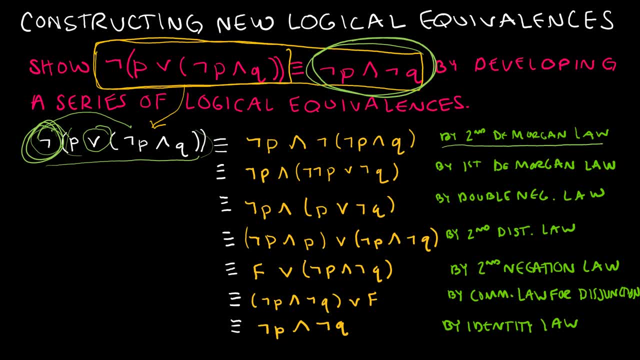 again. why did I do that? Because I don't like this negative hanging out there on the outside. Now I'm going to continue and I've got a negation on the outside of an and statement, And so I'm going to continue. and I've got a negation on the outside of an and statement, And so I'm going to. 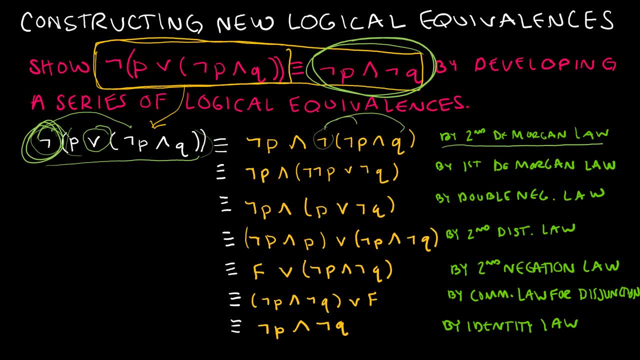 use the first De Morgan's law that says if you have the negation on the outside, it's going to distribute to both and turn it into an or statement. So that's all I did for my second step. Notice what I'm doing is I'm writing the result and then writing the reason why. 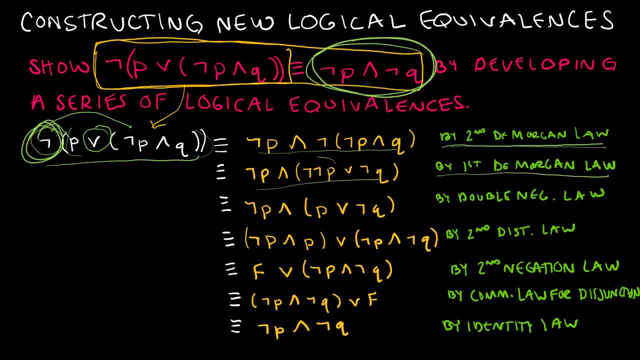 Writing the result and then writing the reason why. Now I'm looking at the fact that I have a not not p, So I'm just changing it to a p by the double negation law. And then I'm looking at I've got not p, and, and then I've got a compound proposition And so I'm going to distribute. 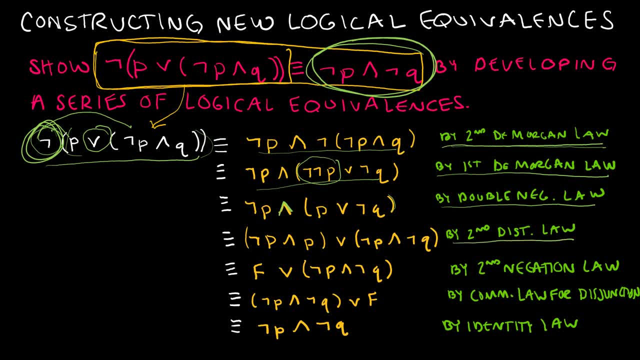 that not p by the second distributive law. So I'm taking not p and p or not p and not q. Now I'm replacing not p and p with false, because we know by the second negation law that if we have not p and p that it must be false. It is a contradiction. 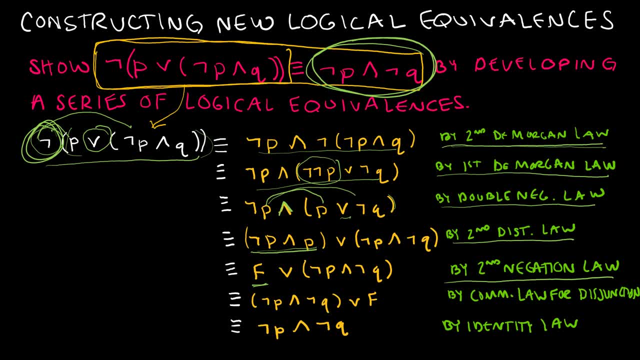 Now I have to switch the order, which is what I did here, by the commutative law for disjunction, And I'm okay if you just write the commutative law, It says commutative law for disjunction, because obviously we're dealing with an or which is a disjunction, And the reason that I did that 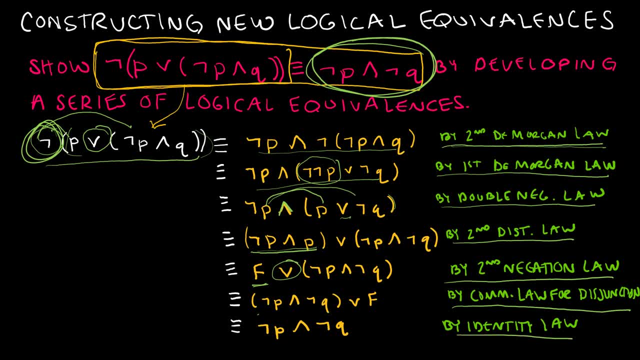 is because the identity law is written in this format, with the false coming second, And so we have to put it in that format to use the identity law. The identity law says: if you have something or false, it's whatever that something was. And so notice now. 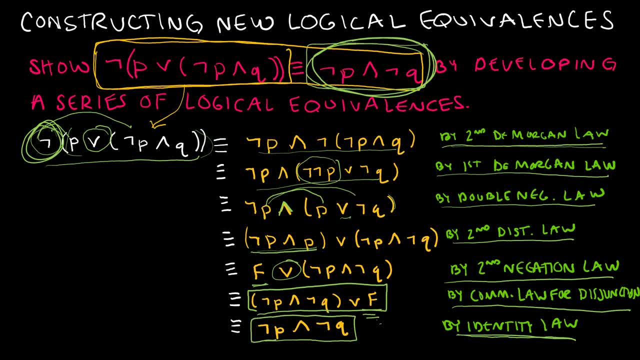 I've ended up here at not p and not q, which is where I wanted to end up. So we showed this with a truth table and show that it was in fact logically equivalent. But now this is just a little bit, I guess, more secure way to do it, because we're using all of our known identities. 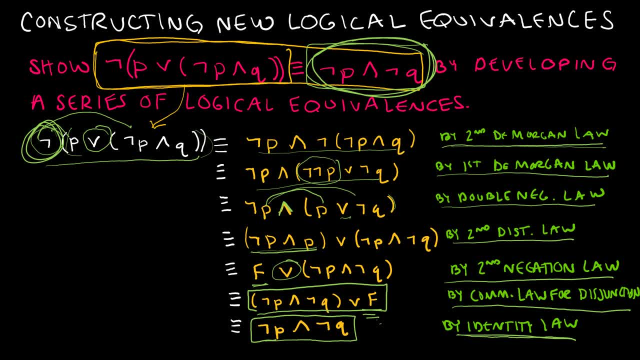 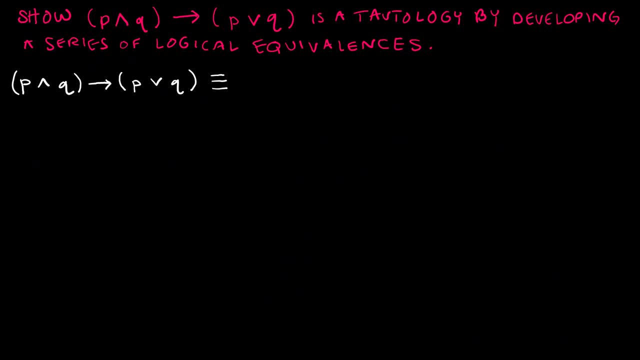 or known laws that we can use with logical equivalences. In this example, we are trying to show that if p and q, then p or q is a tautology, And again we're going to use the same method that we just used, But what we're doing is essentially we're 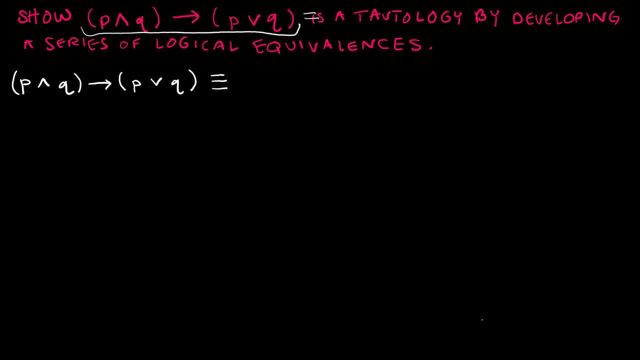 saying: show that all of this is equivalent to true, because, remember, that's what a tautology says- is that it's always true, So typically it's going to give us something on the side. but because it said tautology, that means, whatever steps I go through, I'm going to be able to do. 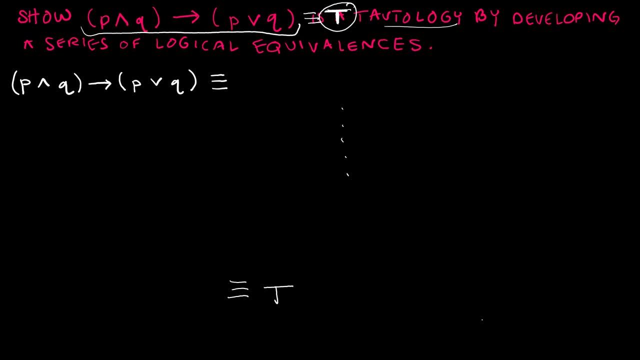 that. So let's see if we can start working our way through this. The first step I'm going to take is a law that doesn't have a name, So we have some laws that talk about if, then statements and different ways that we can rewrite them, And one of the ways to rewrite them is that if p, then q. 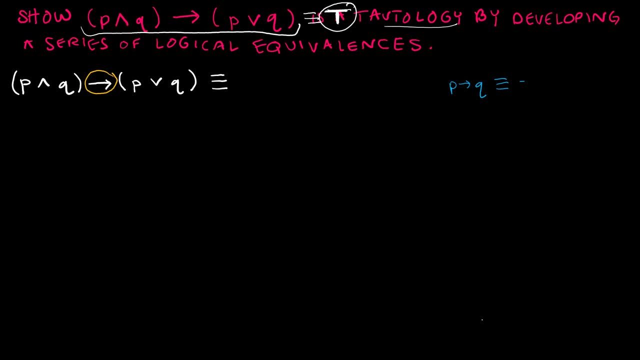 is equivalent to not p or q. So that's what I'm going to do, is I'm going to use that law to say not p and q or q, which is p or q, Because, remember, p and q here are compositional compound propositions. So that's all I've done is. 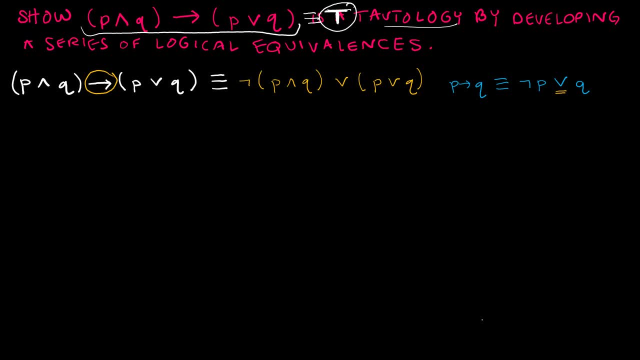 I've applied that rule, So step one done. Then I'm going to say, okay, well, that is the same or equivalent to not p or not q, And then notice the stuff on the right side. I'm not changing. 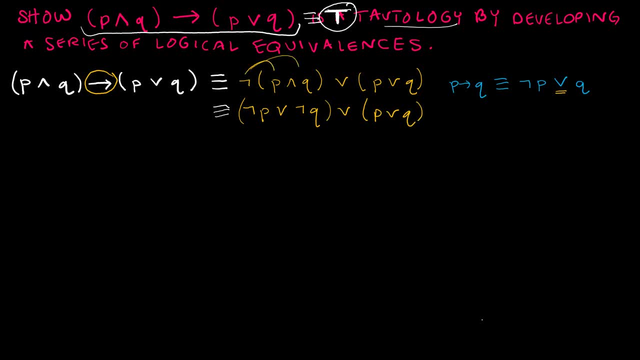 Now, how am I able to do that? Well, all I did was distribute that negation. remember, when we're distributing negation, we're dealing with De Morgan's laws, and that is the first De Morgan law. Now I'm going to say, well, I've got a, not p, and a, not q, and a p and a q. 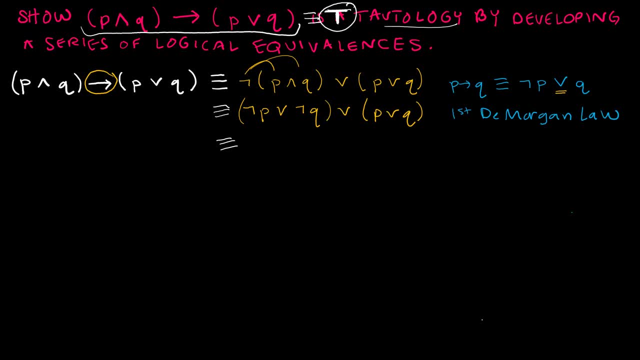 So I'm going to do some rearranging. Now I could. the rule is you should only do one thing per step, But because it's all kind of the same thing, I'm just going to do one thing per step. So I'm going to do some moving around and regrouping, So I'm going to rename this. 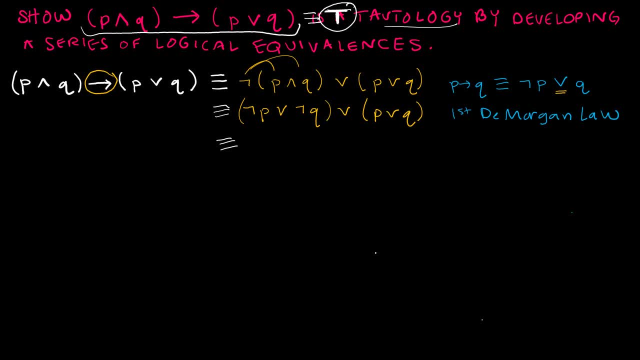 whoops, let's keep the same colors here. I'm going to call this p or not p, or q or not q, And again, I did quite a few things here, but it's sort of simple things, So it's things that are easy to follow. So again, 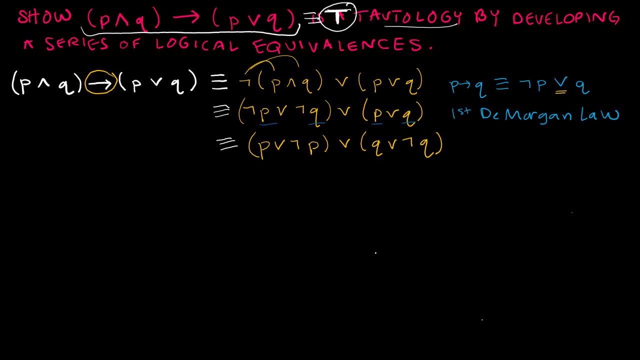 I had a P and a not P, a Q and a not Q and notice these were all ors. So what did I do? I used the commutative by changing the order and associative laws for disjunction. So disjunction because I've got all of the ors and it's commutative and associative. 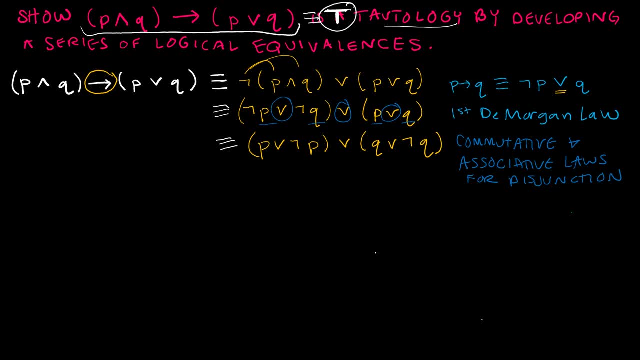 because I switched the order and I grouped them differently. Okay, so now I'm going to say that I've got P or not P and a P or not P is true, and I'm keeping that This the same. Whoops, I keep switching my colors. 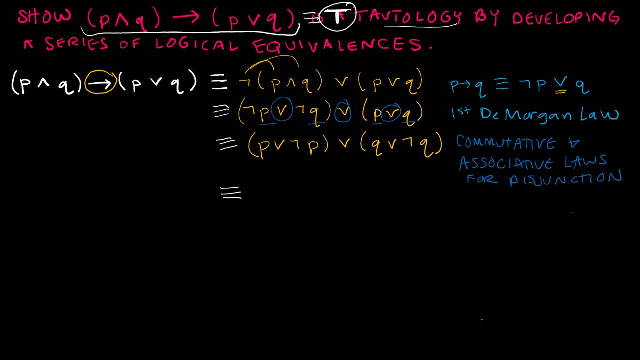 Darn it, Hold on a minute, Let's do that again. So P or not P is true, or Q or not Q is true. and I'm doing those both on the same step because it's the exact same law and that law is the negation law. 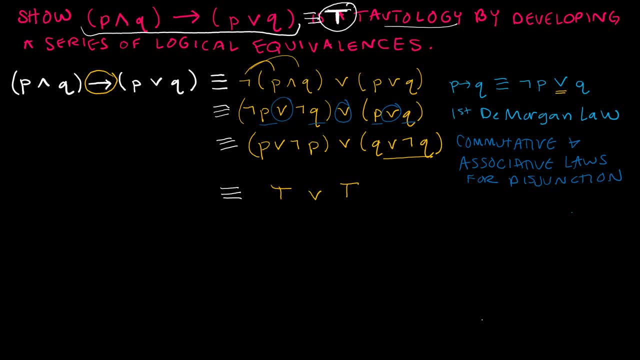 Or I believe that's actually the second negation law. Now I'm not so worried about naming the first or the second, except for the De Morgan law. you really should say if it's the first or the second. But if you just said the negation law on that one, I would be just fine with that. 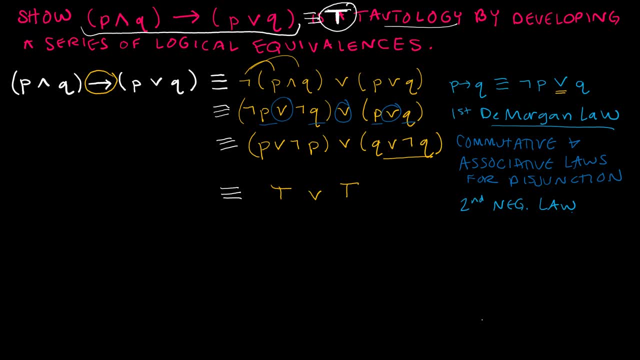 So now I have true or true by the second negation law, and if I have true or true, then I can say that that is in fact congruent to true. What rule can I say is saying that it is congruent to true? and that is the domination. 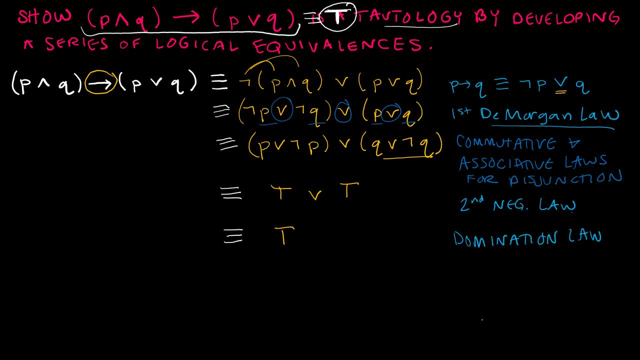 law because, if you'll recall, the domination law says P or true is congruent or equivalent to P and, of course, if this is true or true, it's congruent or equivalent to true. So that is how I would prove that. 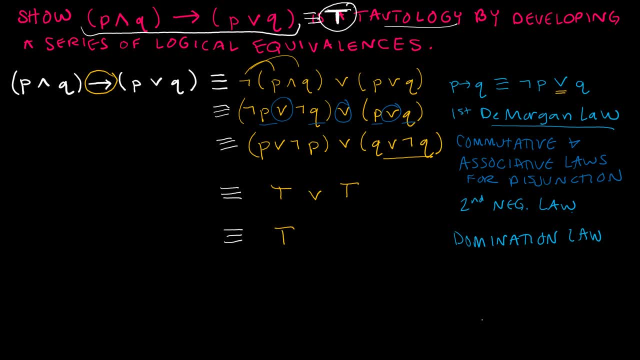 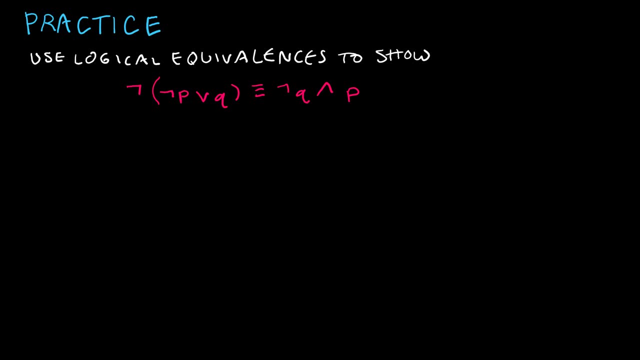 Again by developing a series of logical equivalences. Here's one for you to try on your own. So if you would press pause, try this question and when you're ready, press play to see how you did. As always, I'm going to start by writing whatever is on the left side. 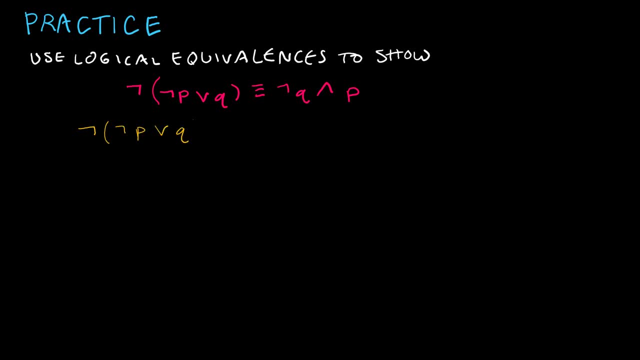 So I have not not P or Q, and then I'm going to perform whatever. my first step is keeping in mind that this is my goal. So the first thing I see is I have a negation on the outside of a compound proposition and that, to me, just screams De Morgan's law.